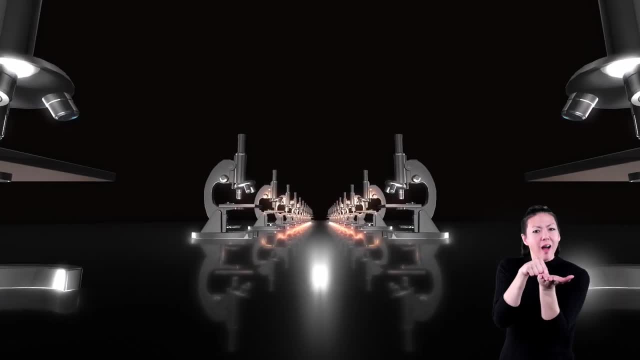 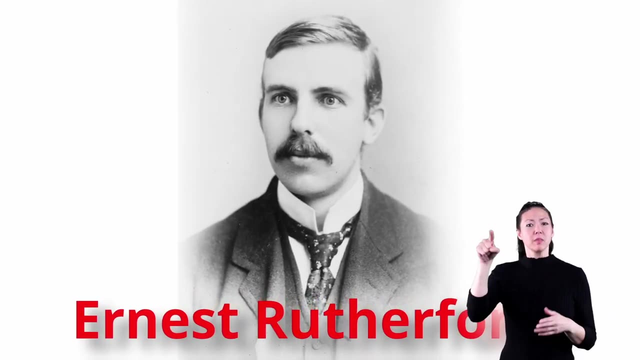 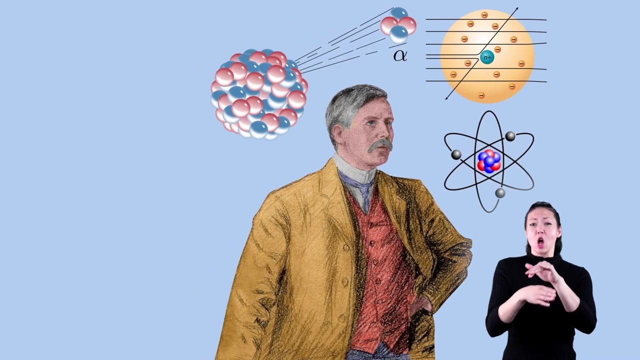 see them with the highest powered microscopes, But we do know they're there. That's because more than a hundred years ago, a scientist named Ernest Rutherford was able to bounce other small particles off of atoms and witness the interaction. It was kind of like you bounced a soccer ball off a tiny, tiny super ball. The way that super ball 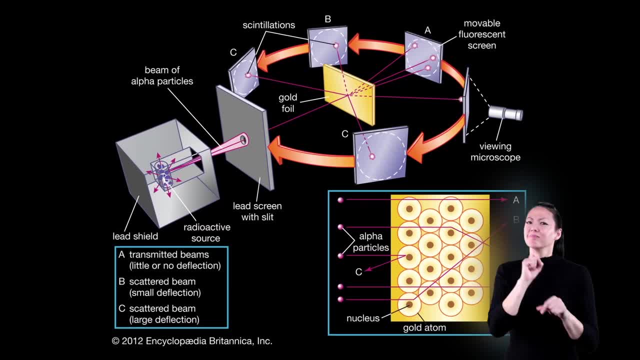 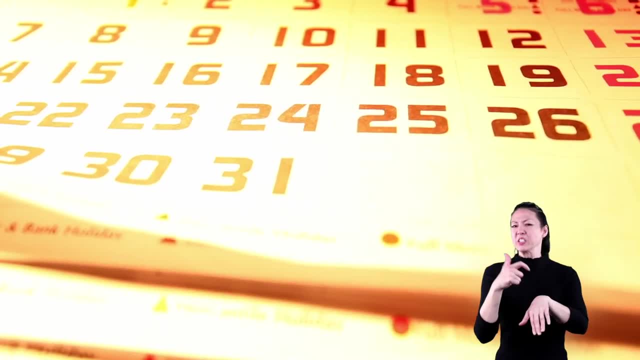 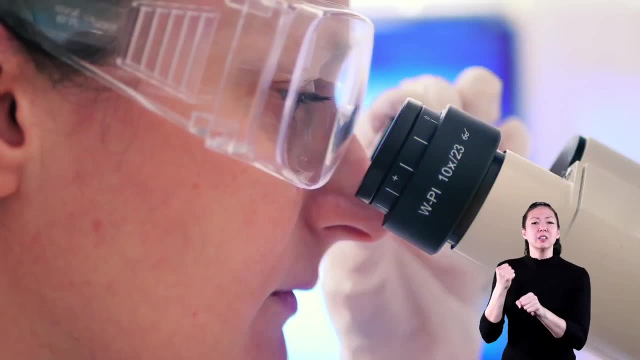 or, in Rutherford's case, atoms acted, told him they existed and what they were made of. This history of how atoms were discovered is a lesson for another time, But scientists have proven the existence of atoms in many different ways over the last century. They're definitely 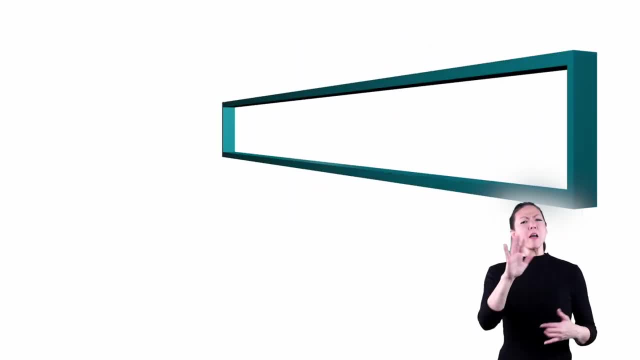 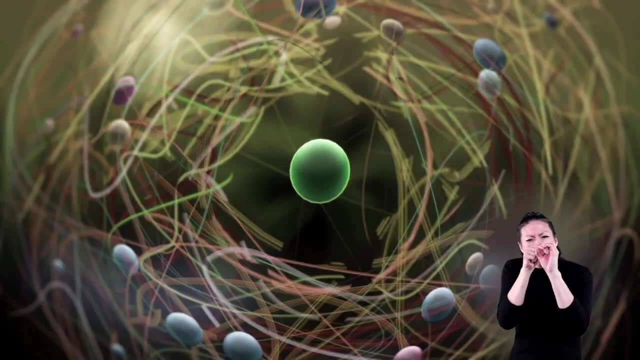 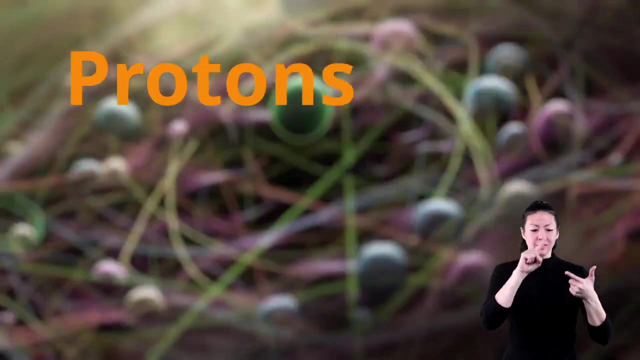 there And they're really cool. So what is an atom made of And how does it behave? So how is an atom made of? It's hard to believe that inside every atom there are three even smaller particles. These particles are known as protons, neutrons and electrons. The difference in the way these 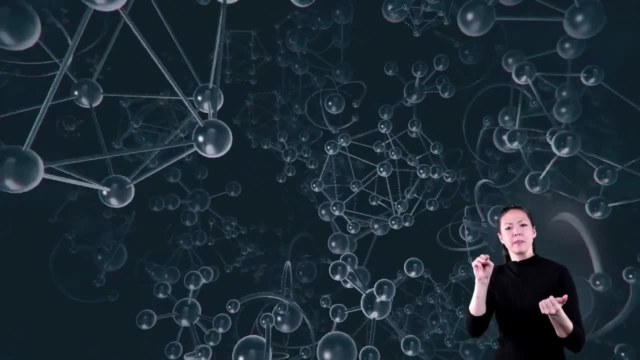 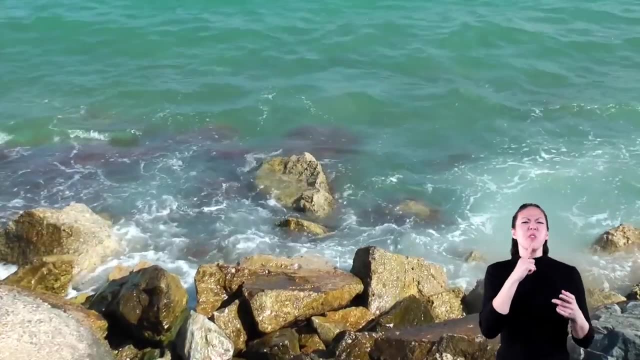 three particles exist within every atom, and the ways they interact with other atoms helps determine what these atoms create. These atoms make up why we live up wood or water or metal or anything. But we'll get to that shortly. First let's 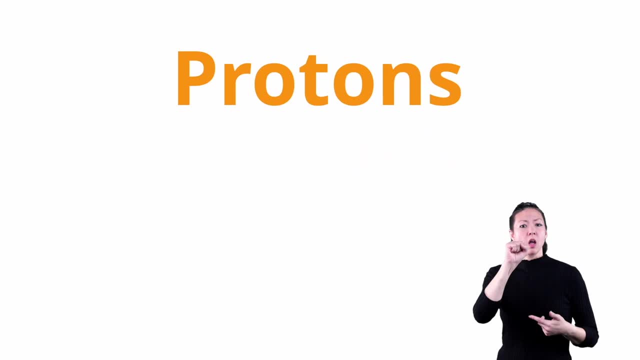 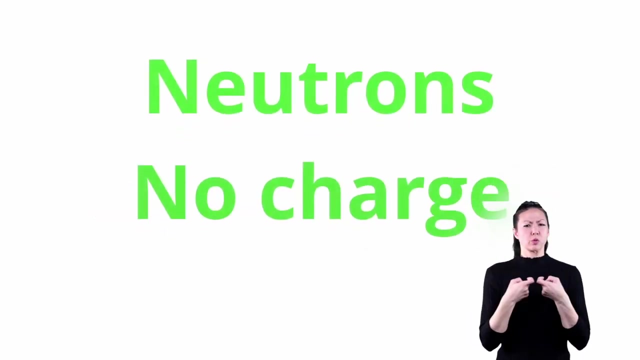 talk about these three particles: Protons, neutrons and electrons. A proton carries one unit of positive electric charge, An electron carries one unit of negative charge And a neutron has no electric charge. Together, the protons and neutrons make up the nucleus. 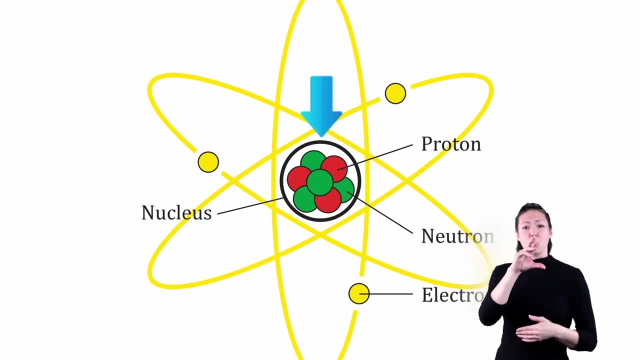 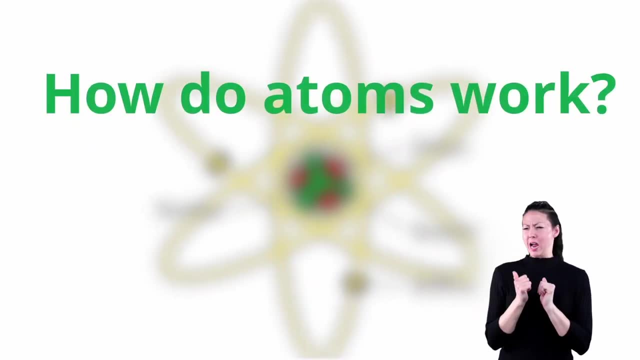 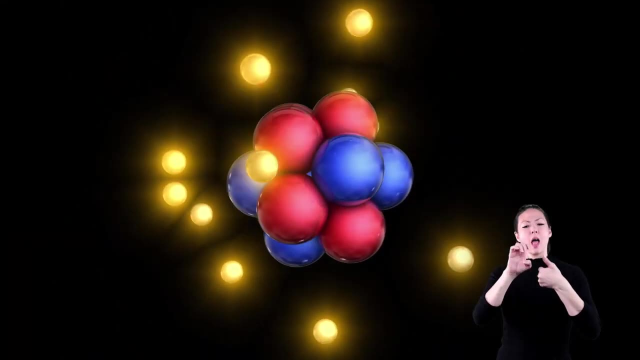 of an atom or its center, And the electrons spin around the outside of the nucleus in what is called a shell. How do these super tiny atoms work And what do they do? The different ways that atoms are organized determines what they are or what elements they make. 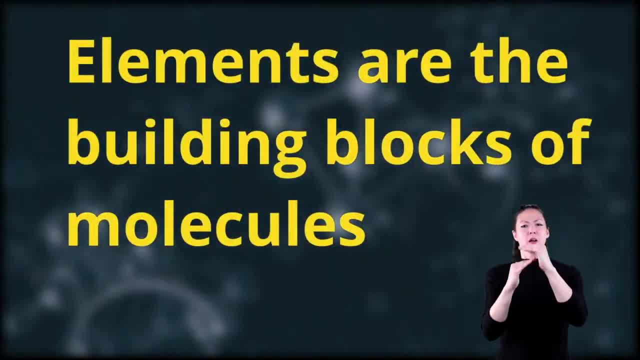 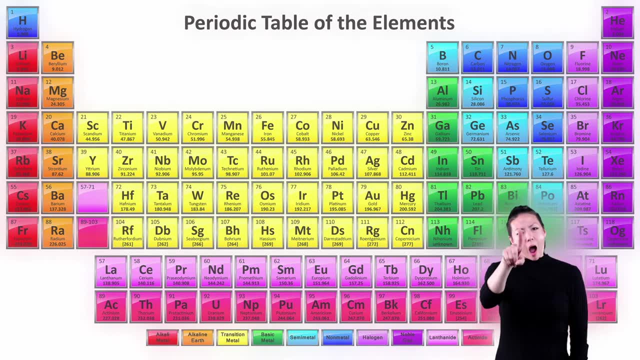 up. Elements are the building blocks of molecules And everything around us consists of molecules. All the elements are different and there are a hundred and twenty of them. These hundred and twenty elements are laid out here in the periodic table of elements. This chart is used by scientists like physicists and 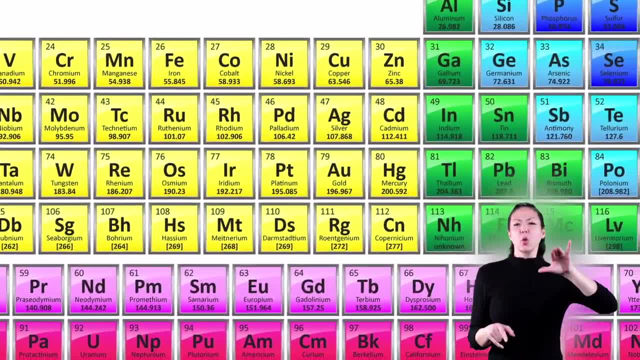 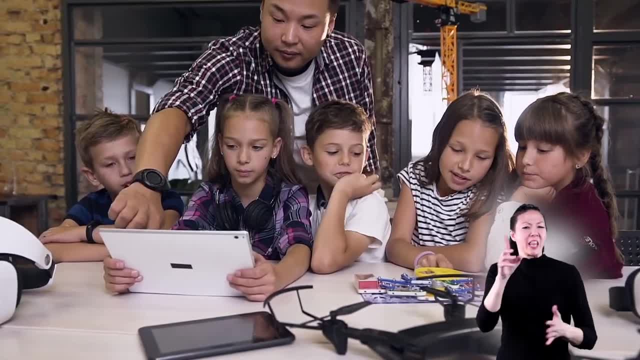 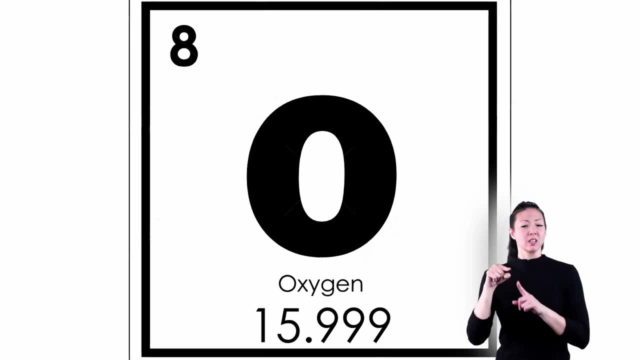 chemists to study how solids, gases and liquids behave. It all depends on what they're made of. You'll probably spend a lot of time studying this chart later, but it's very useful as you continue learning about science. This is the element oxygen. The number eight means that the atoms that make up oxygen have. 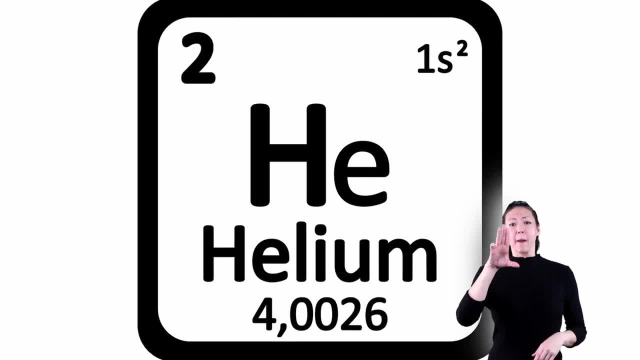 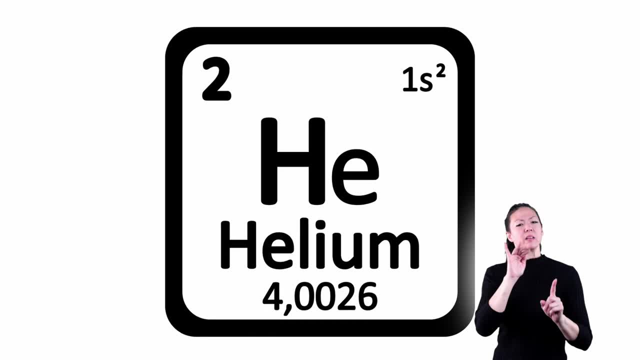 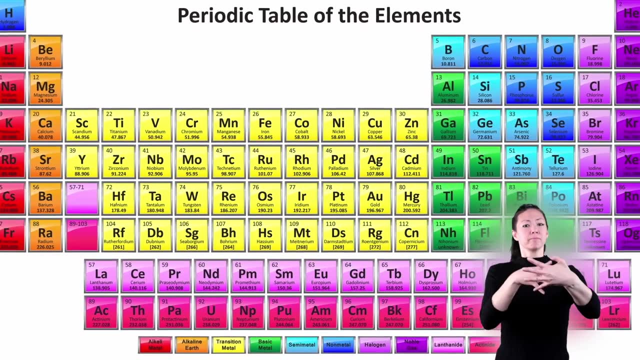 eight protons. This is helium, and its atoms have two protons. The number at the bottom tells us what the atomic weight of the element is. As you can see, there are a hundred and twenty such elements on the periodic table, And each 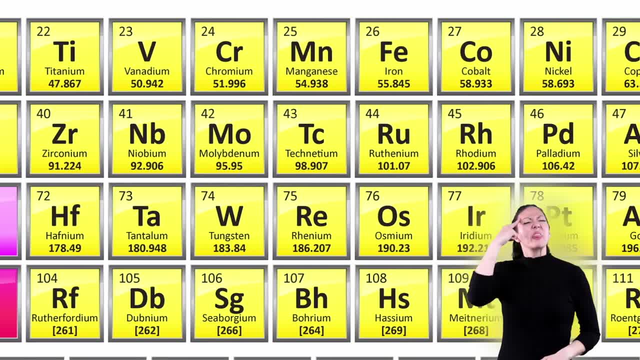 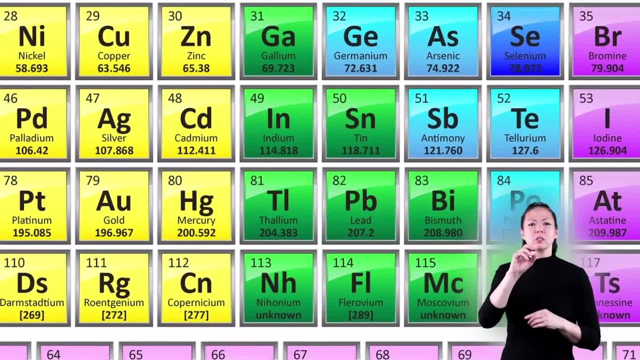 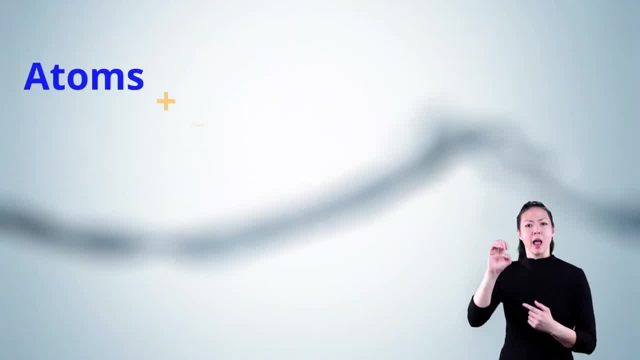 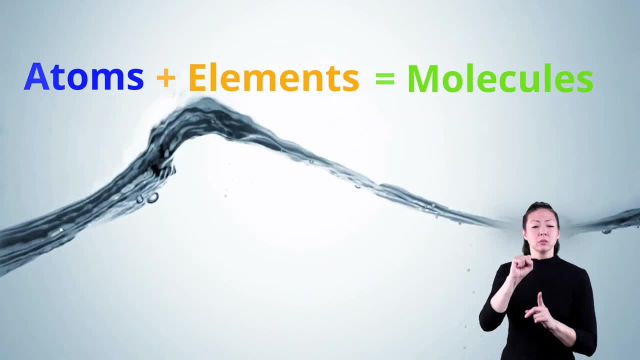 the word is the number of protons, neutrons and electrons that make up the atoms in an element. tell you what the element is, And when atoms and elements are joined together, they make up molecules. Water, for example, is a molecule. Each water molecule is made. 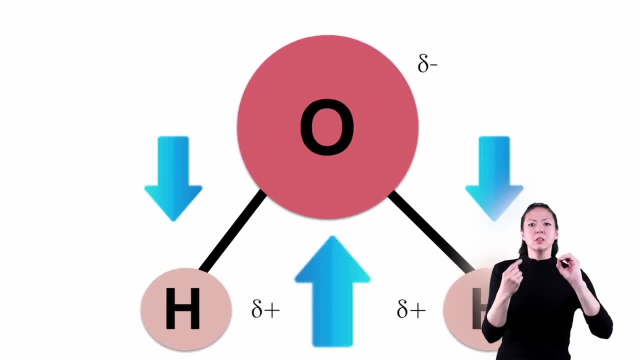 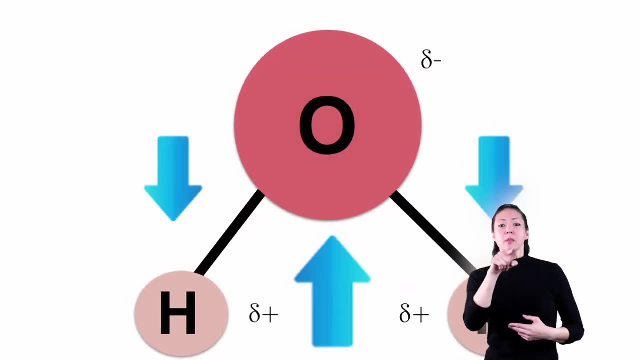 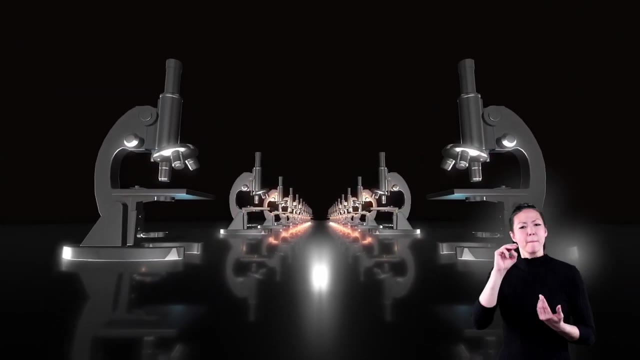 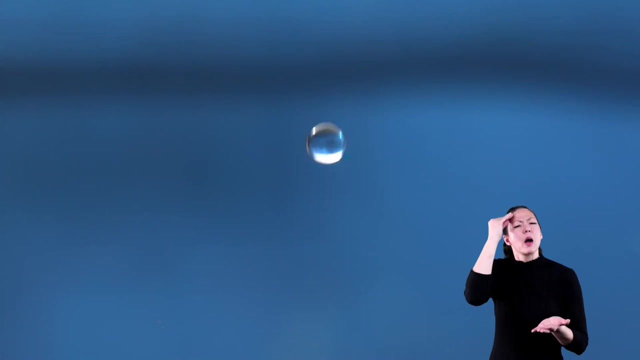 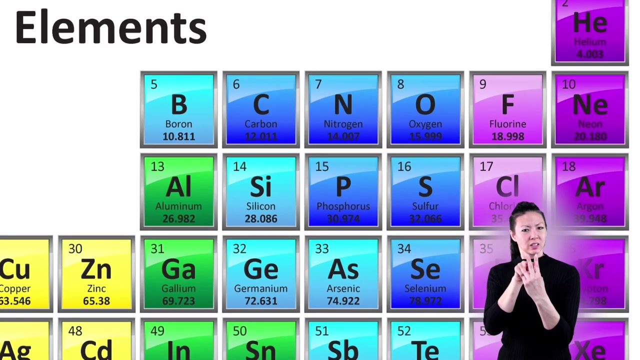 up of two hydrogen atoms and one oxygen atom. Hygiene, oxygen and water all commit to oxygen. Hydrogen and hydrogen are polycyclic atoms, but they play a significant role in the adaptation of water, And within those molecules are even tinier atoms of hydrogen and oxygen. 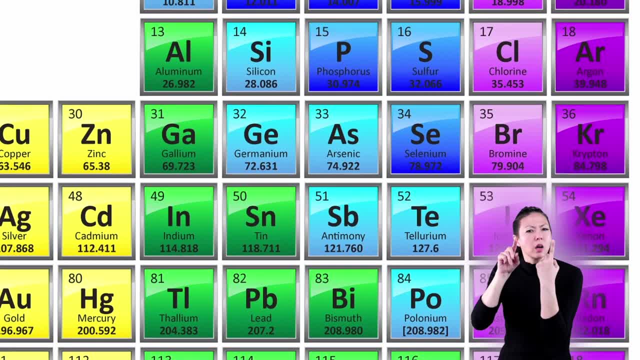 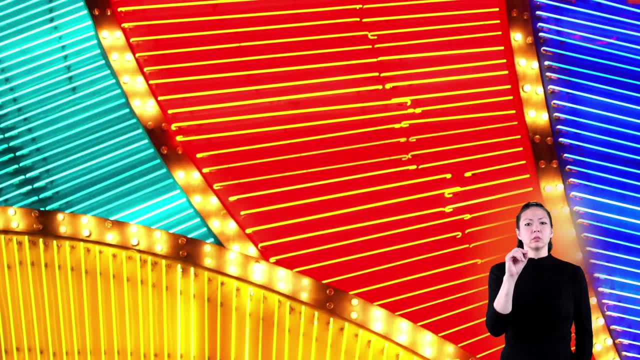 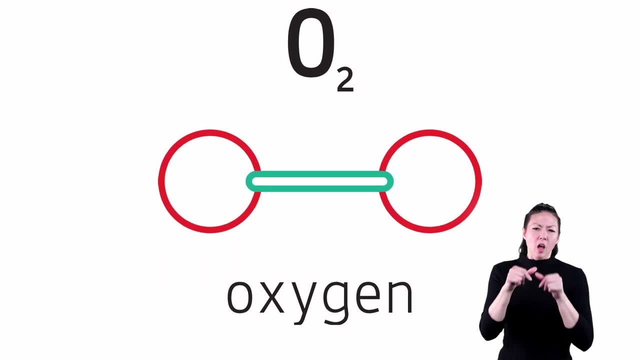 Some elements are actually made up of a single atom that doesn't attach itself to other atoms. The element of neon is one such example. It has just one atom, But other elements are made up of more than one atom, like oxygen, which usually consists. 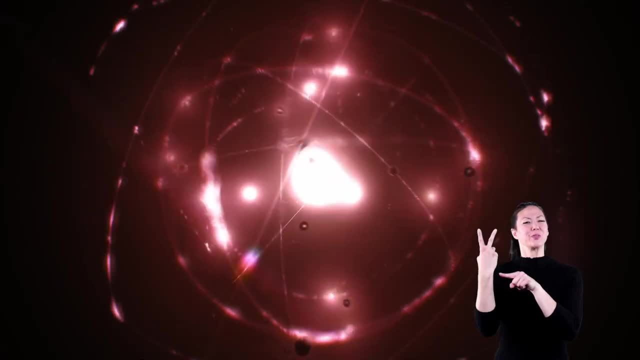 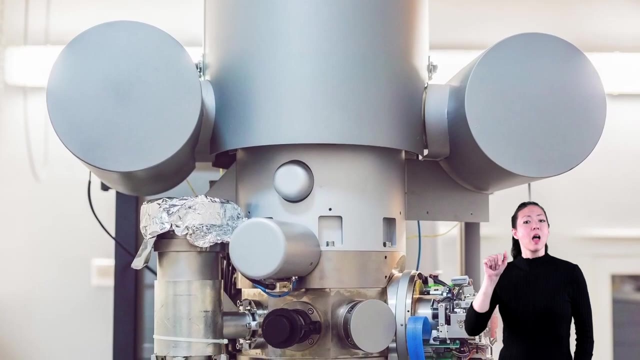 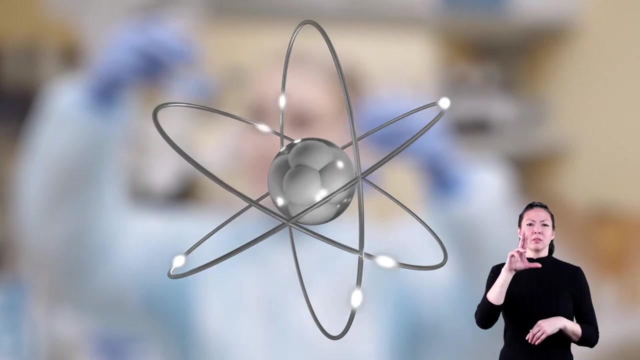 of two. It's referred to as O2.. So to sum up, try to think of all the things around us as a recipe of atoms. Atoms are incredibly tiny and consist of a certain number of protons, neutrons and electrons.